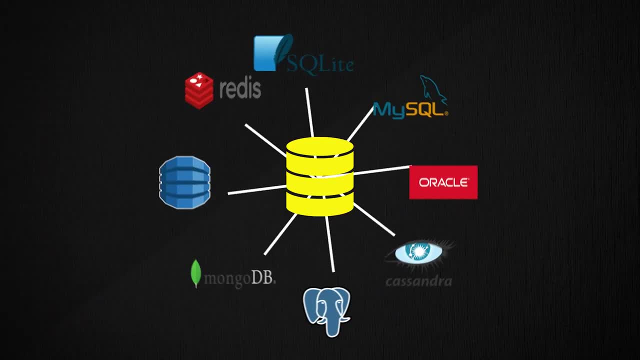 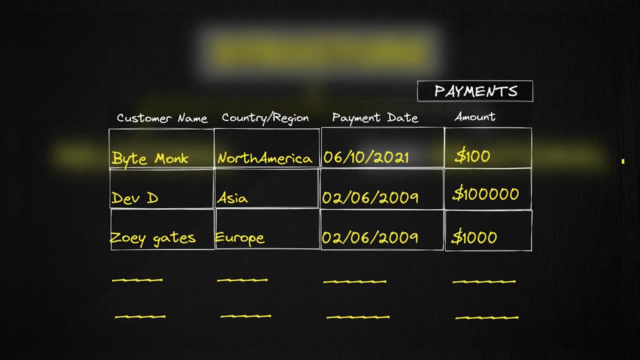 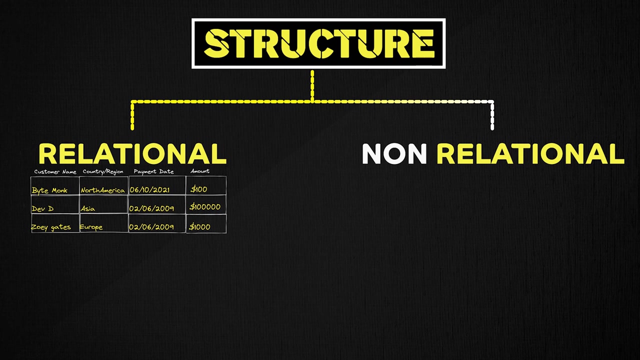 it is quite similar to a dictionary or a map data structure. Now, in one of my previous videos in System Design Playlist, we learned the benefits of structure, which relational database imposes because it gives us very powerful and complex querying capabilities. However, depending upon the use case, the same structure can be more cumbersome than useful. 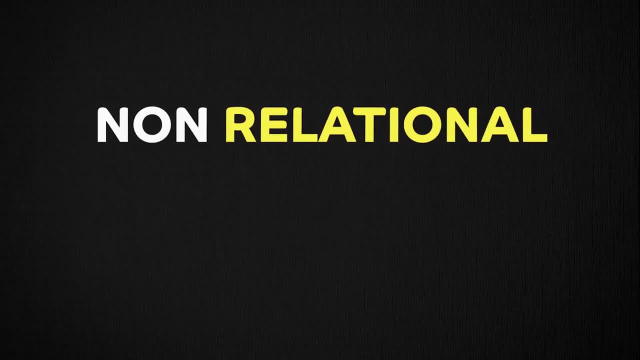 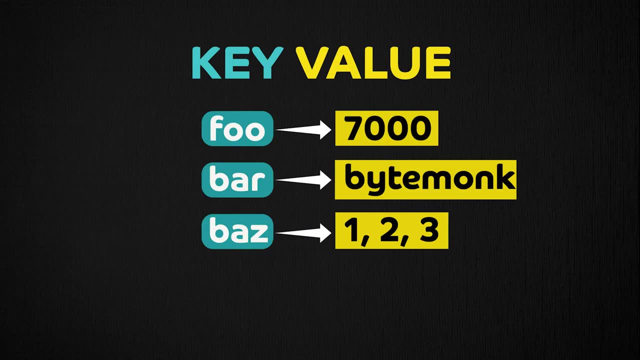 And in those cases you may prefer to use a non-relational or NoSQL database, that is, a database that does not need any tabular-like structure. Key-value store is one of the most popular types of non-relational databases, As its name implies. a key-value store is a database that allows you to store mappings from. 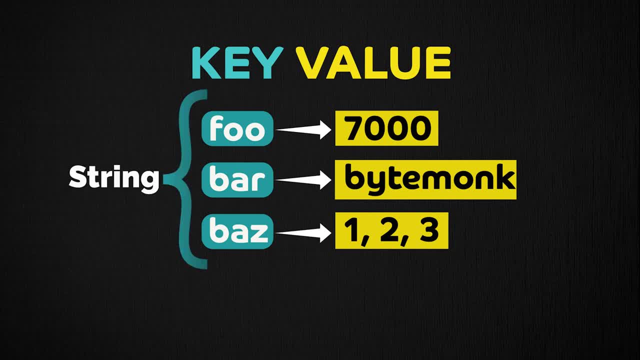 keys which are typically strings to arbitrary values. These key-value stores can be used to store keys which are typically strings to arbitrary values. These key-value stores can be used to store keys which are typically strings to arbitrary values. 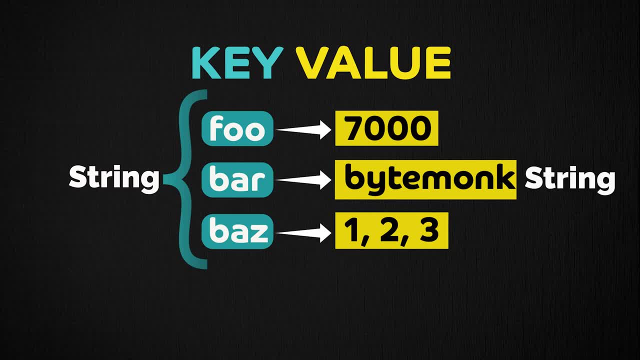 These values are typically also stored as strings, but some key-value stores will also allow you to store integers or arrays as values. Key-value stores can be considered as the most primary and the simplest version of all databases. It just has one-way mapping from the key to the value to store data. 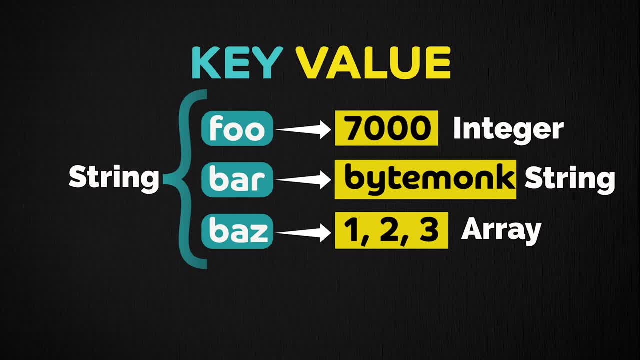 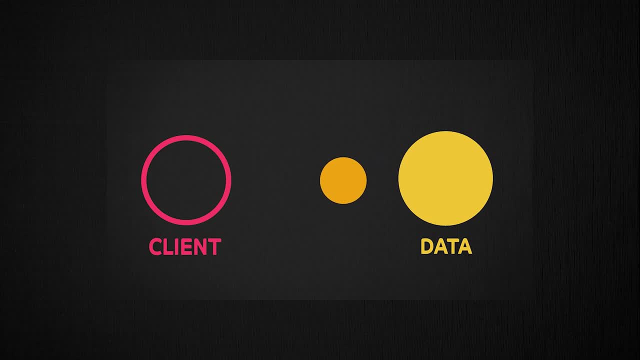 The lack of any imposed structure makes them extremely flexible. For example, if you think about caching, it's a perfect candidate for a key-value store, because when you implement caching, you are typically storing values somewhere and access them using a hash, a username or IP address. 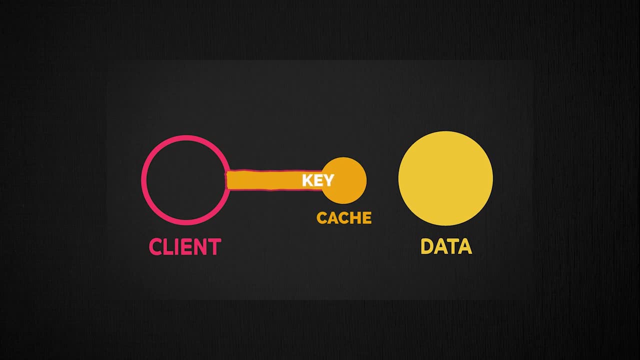 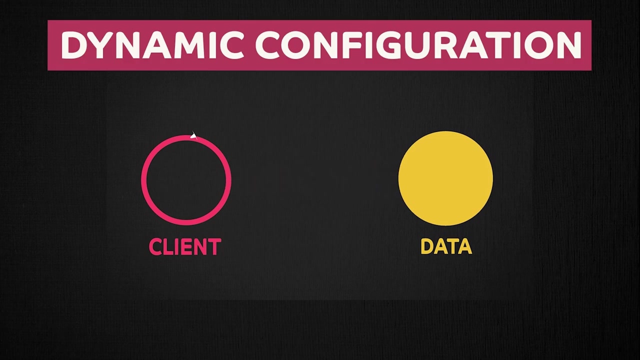 Basically, you access them using some sort of a key. Conceptually, you are using a key-value model, and so key-value stores are typically the databases used for caching. Redis is a popular example to implement caching. Another example that comes to my mind is of dynamic configurations. 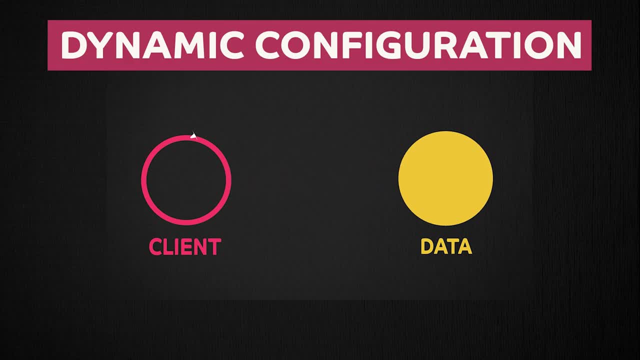 which I will cover in another video. but to explain it briefly, sometimes you may have special parameters that different parts of your system may rely on. For example, I might like to store a value in a database indicating if my system is up or not, So I can have a parameter like isLaunched and a 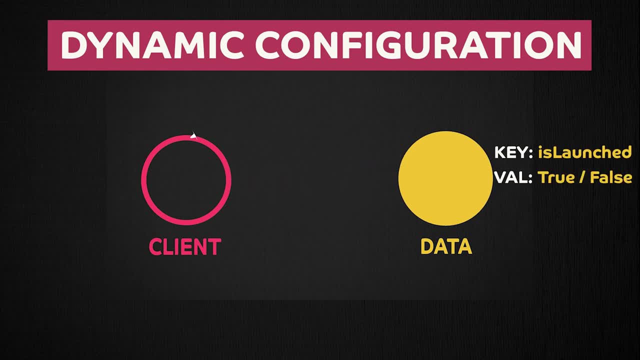 boolean value true or false, determining if the system is launched or not. Since you are accessing values directly through the keys, you don't have to search through the database sequentially, one by one, going through every entry. You can just access them directly using keys, which makes them 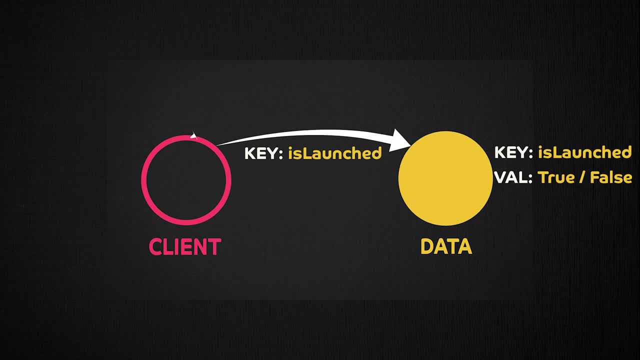 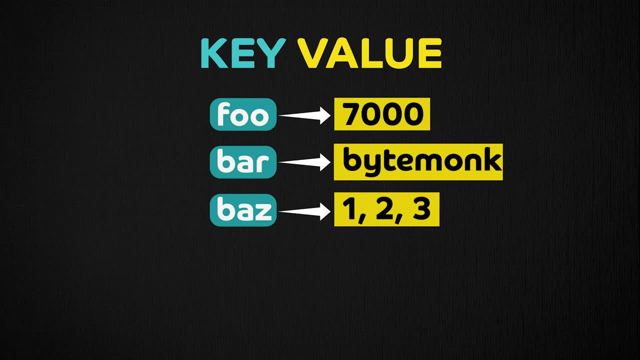 extremely fast, and so you will always be able to access them. You will often get low latency and high throughput when using key-value store. At the same time, key-value stores usually do not have a querying language as in RDMS. to retrieve data, They only provide some simple operations, such as get, put and delete. 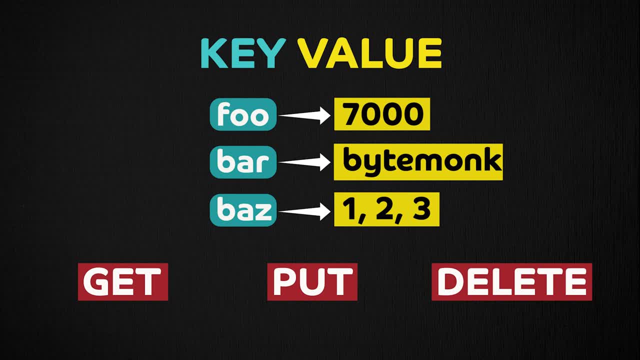 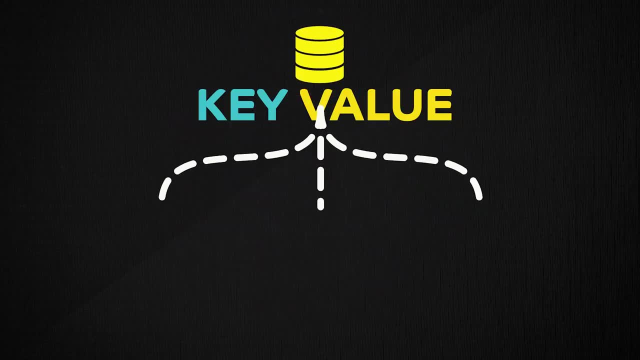 Hence the data querying or retrieving should be handled manually at the application level. Now there are a lot of databases out there and naturally there are various types of key-value stores, For example, DynamoDB, Redis, ZooKeeper and different key-value. 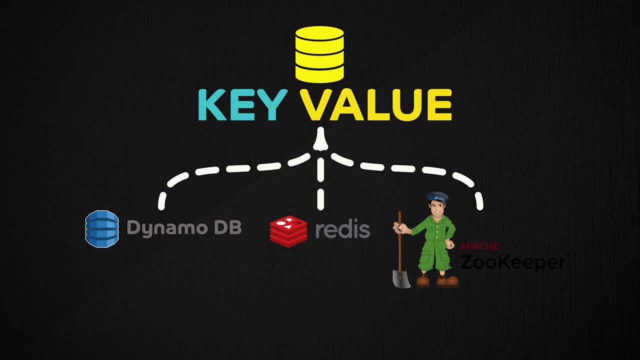 stores may behave differently. Some key-value stores, such as DynamoDB, write data to disk, meaning the data will persist even if they crash or go down. Key-value stores such as Redis might only write data to memory and if they crash, you will lose the data stored in them. This is 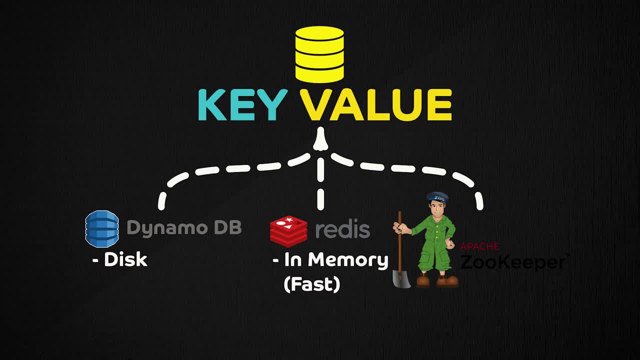 a trade-off. you make for faster operation which, depending upon your use case, might be totally acceptable. For example, if you are using a key-value store for caching and you lose your data, it might not be unacceptable for your system. All you will miss is a few cache hits and once your key-value store 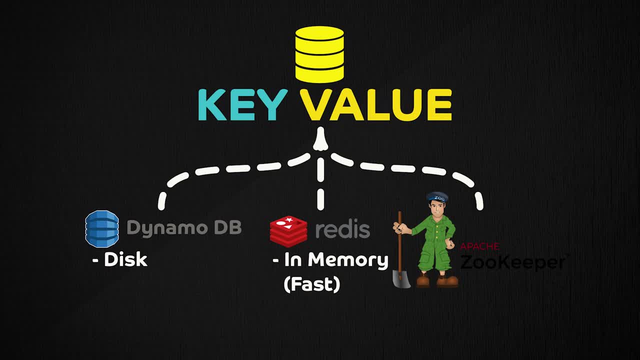 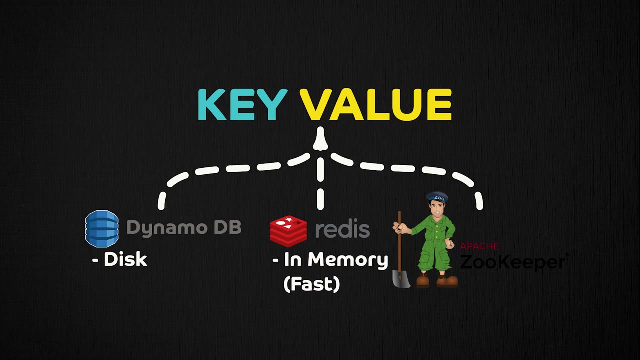 is back up, you will start refilling the cache and those cache hits again. Some key-value stores will give you strong consistency. Some will give you eventual consistency. The point is there are a lot of key-value stores out there and you have to pick the one that's going to be most useful for. 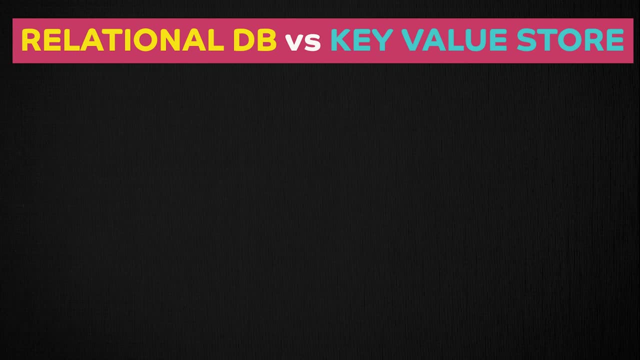 the use case you're dealing with Now. there is absolutely no reason to use a key-value store over RDBMS for a simple, typical business-based application where data management is more important than the performances. But if your application is more performance-driven, 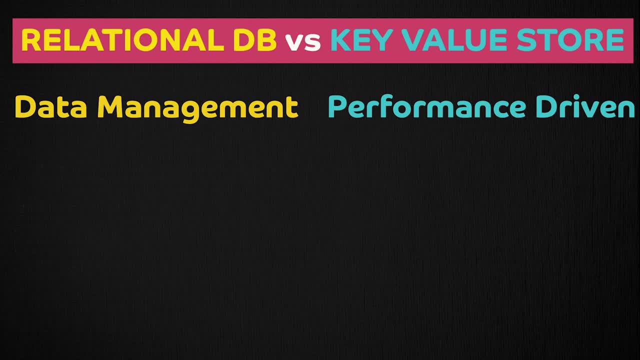 you should certainly use a key-value store over RDBMS, since the key-value stores are capable of providing much higher performance than RDBMS. Also, if your data model is not hierarchical, you should consider using key-value stores over RDBMS, As the key-value stores are really simple. 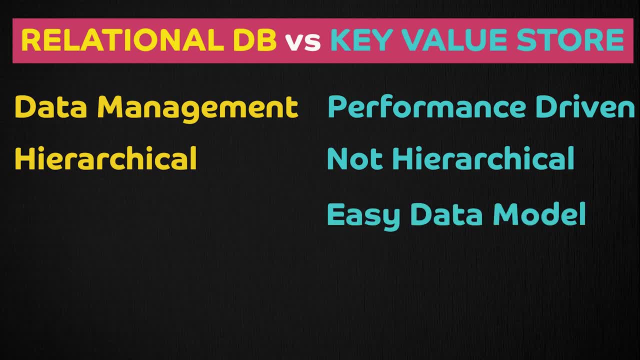 and easy to handle. data can be modeled in a lot of different ways, For example, if you are using a less complicated manner than in a RDBMS, and it will end up having much better performance than RDBMS, as well. As both of these databases types have their own strengths and weaknesses, you